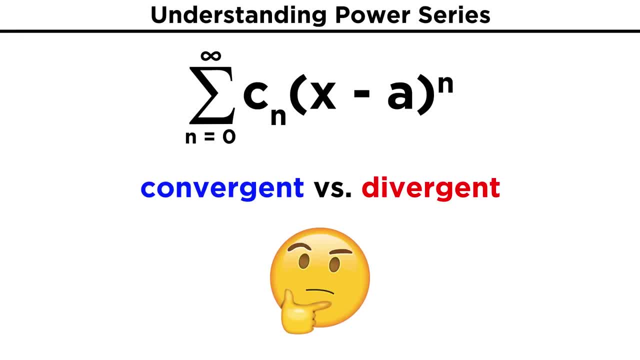 minus A is being raised to the N power. How can we assess whether this kind of power series is convergent or divergent? Sometimes we will use the ratio test. Take something like the quantity X minus three raised to the N power over N. Remembering: 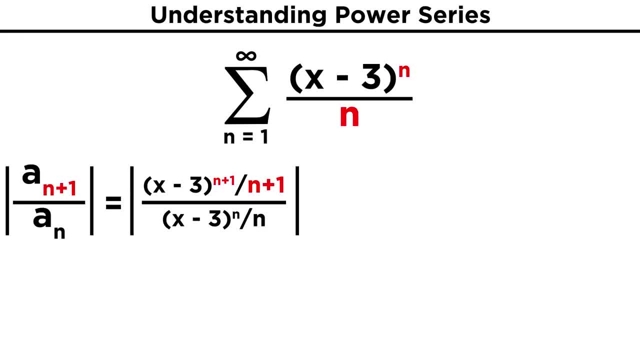 the ratio test from the previous tutorial. let's change N into N plus one and then take the regular version and flip it to bring it up here. To simplify: X minus three raised to the N plus one can become X minus three raised. 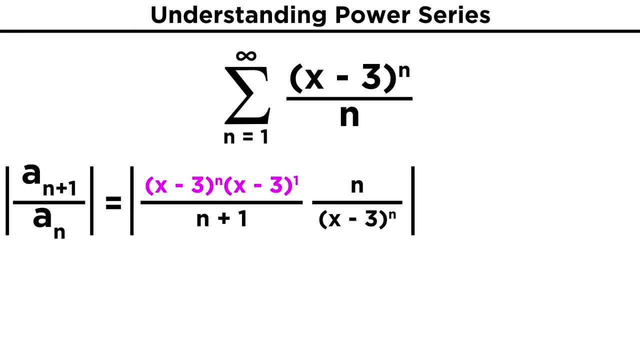 to the N times X minus three. raised to the one, This more complicated term then cancels, leaving us with X minus three times N over N plus one. Now let's divide this fraction by N to get one over the quantity one plus one over. 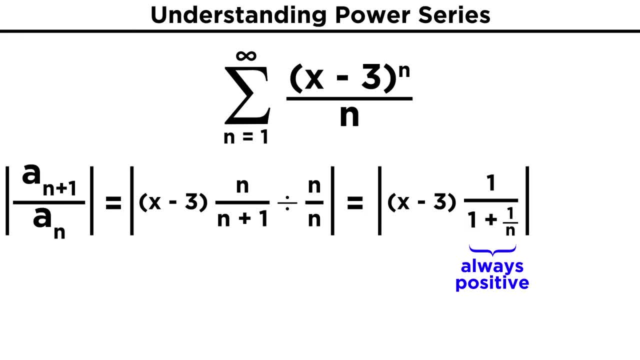 N X minus three raised to the N plus one. As these are all positive, we can pull them out of the absolute value brackets, leaving just X minus three in there Now, bringing N up to infinity. this whole part just becomes one, leaving us with the. 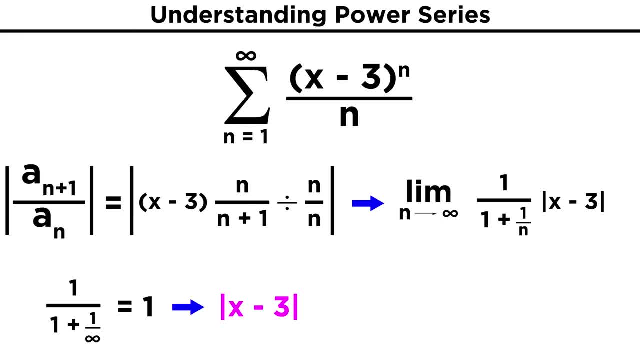 absolute value of X minus three. In order to be convergent, this has to be less than one. so, given the absolute value, we know that X minus three must be less than one and greater than negative one. Adding three throughout, we get X as being between two and four. so those are the values. 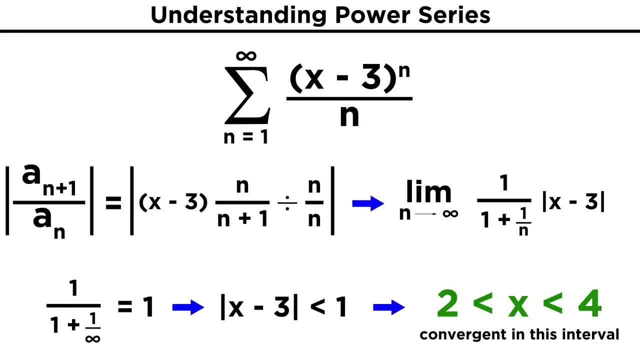 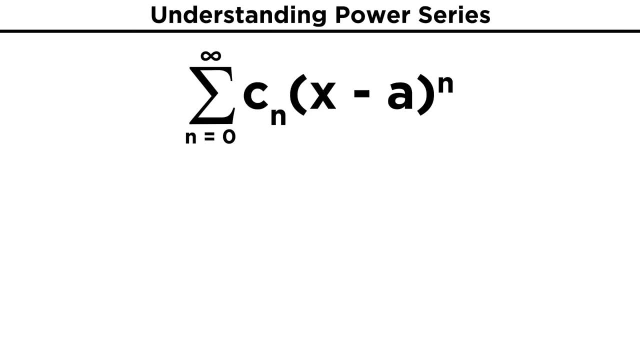 for which the series converges In general. there is a theorem that summarizes the three possibilities that can describe a power series in this form, depending on the precise series. One possibility is that the series converges when X equals A. A second possibility is that 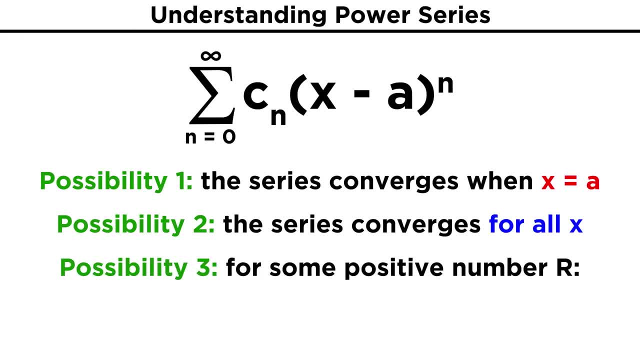 the series converges for any value of X. And lastly, there could be some positive number R, such that if the absolute value of X minus A is less than R, the series will converge and if greater than R, the series will diverge. 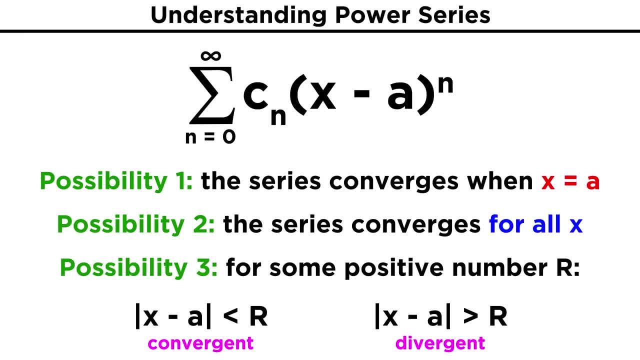 just like the example we just completed In this third case, that number R is called the radius of convergence for that power series. Other cases also involve a radius of convergence. It is simply that for the first case the radius of convergence is zero, as there is. 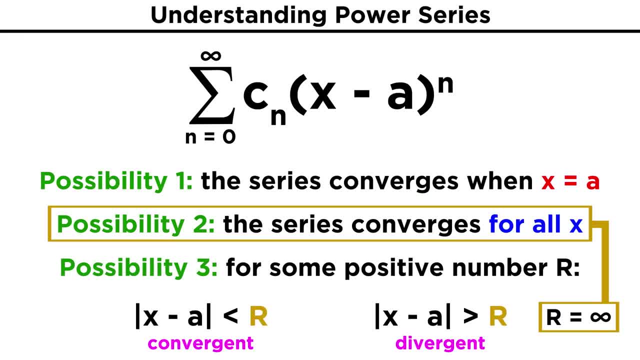 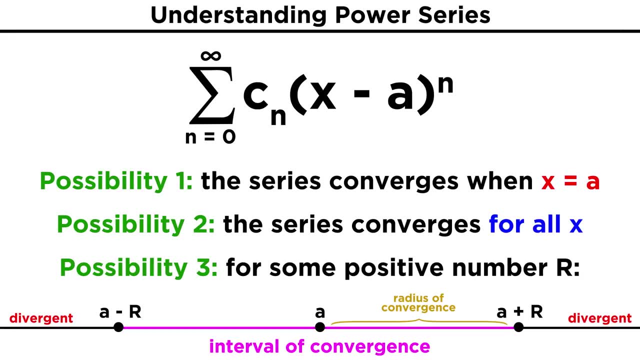 only one value that will allow for convergence, And for the second case, the radius of convergence is infinite, as any value will allow for convergence. We can also describe the interval of convergence as the interval describing all the values of X for which the series converges. 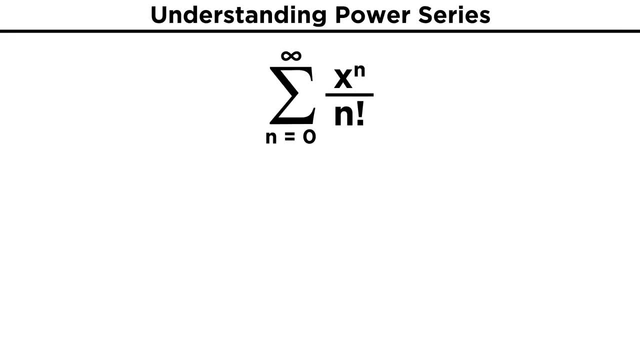 Let's try an example and see how this applies. Take X to the N over N factorial. What can we do with this? Let's try the ratio test. We get X to the N plus one over N plus one factorial, and then given the original series, 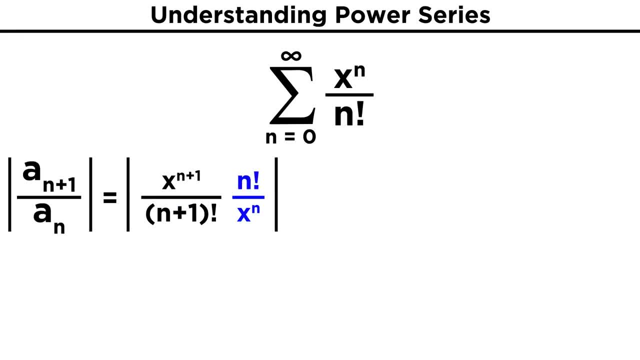 in the denominator. we just multiply by the reciprocal or N factorial over X to the N. We've simplified something like this a couple times by now. so let's change the ratio, Let's change N plus one factorial into N plus one times N factorial, and let's change 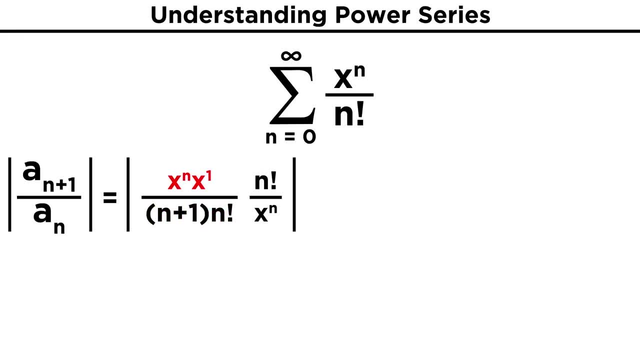 X to the N plus one into X to the N times X to the one. Most of this cancels out and we are left with X over N plus one Finding the limit. as N approaches infinity, we see that we will get zero, no matter what. 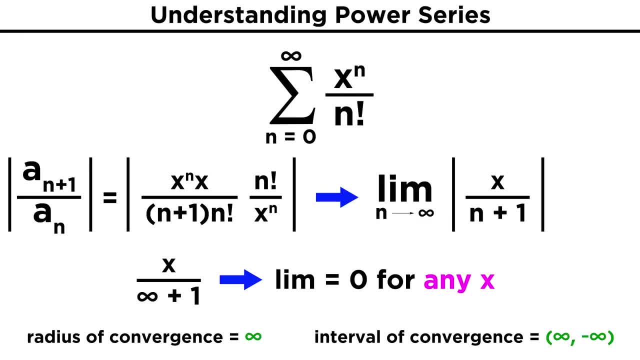 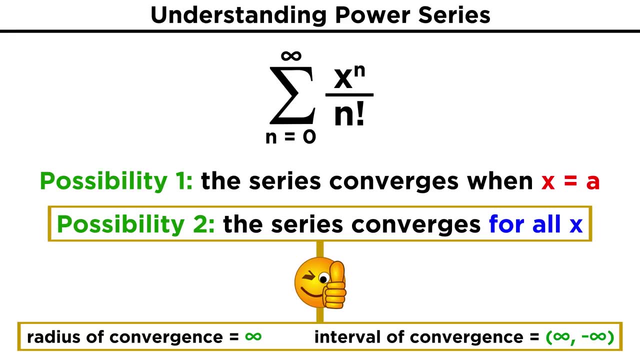 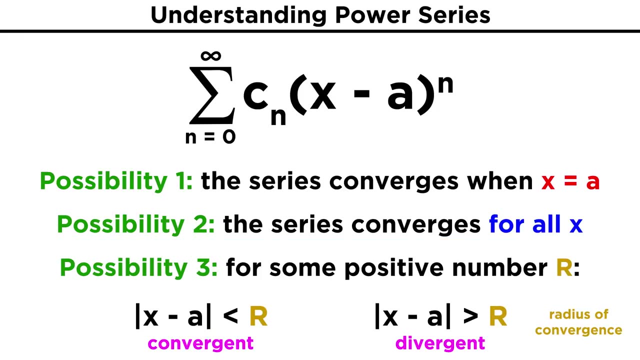 the value for X. This means that the radius of convergence is infinity and the interval of convergence is negative infinity to positive infinity. This fits the second possibility from that theorem, which tells us that this series is always convergent. That covers the basics regarding power series, so let's check comprehension. 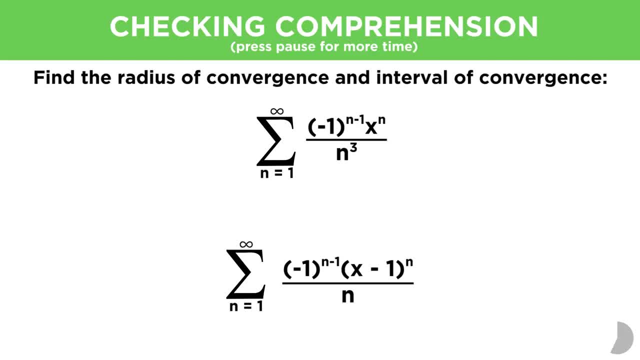 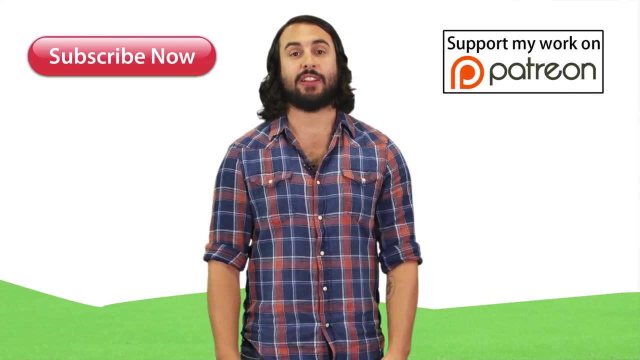 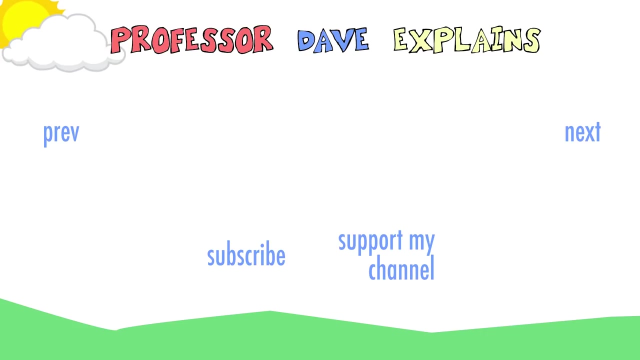 Thanks for watching guys. Subscribe to my channel for more tutorials, Support me on Patreon so I can keep making content And, as always, feel free to email me ProfessorDaveExplains at gmailcom. Have a great day.